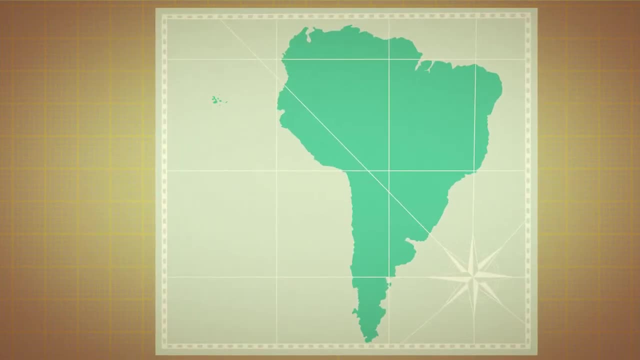 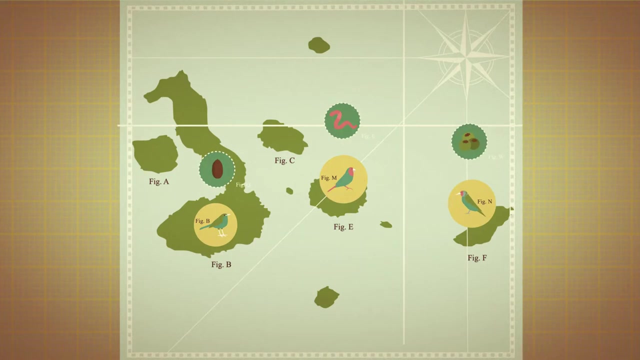 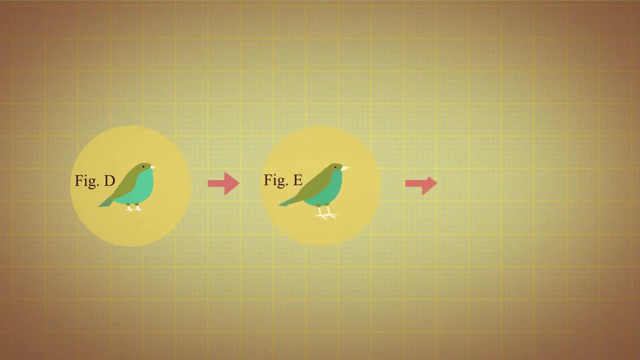 Darwin deduced that when the original finches from South America came to the Galapagos, they migrated to different islands and had to adapt to different conditions in order to get food and survive. These adaptations were passed from one generation to the next. He believed that 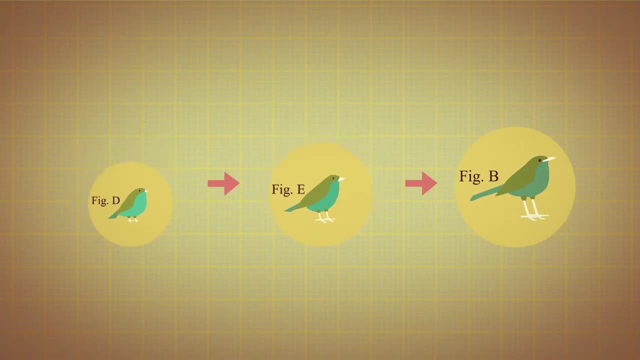 individual members of a species are all similar. Darwin thought that if the traits of the different species were slightly different from one another and that those that are best adapted to their habitat would stand a better chance of surviving, to reproduce and pass on their beneficial traits to their offspring. Over time, those 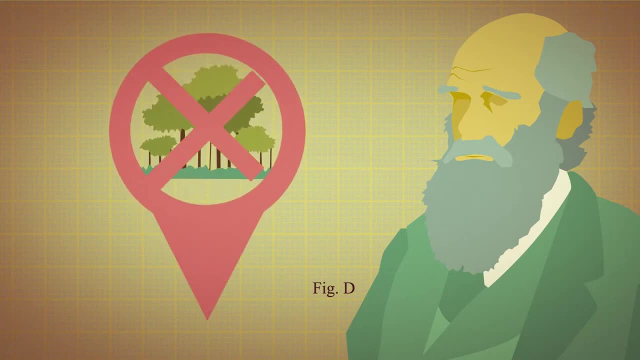 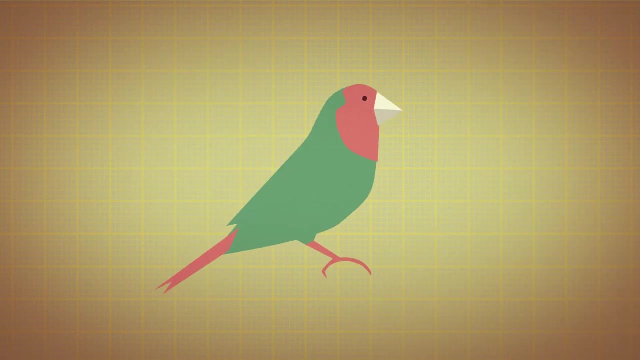 beneficial traits become more common, allowing that particular species to evolve. Critically, Darwin felt that it was not the environment that produced the variations, but chance occurrences to be genetic mutations that enabled an organism to better exploit its environment. After more than 20 years of experimenting and developing his ideas, 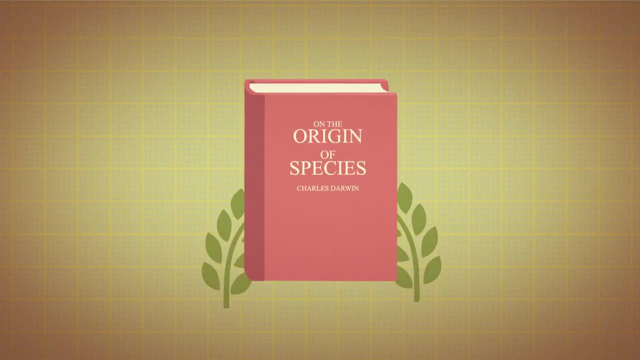 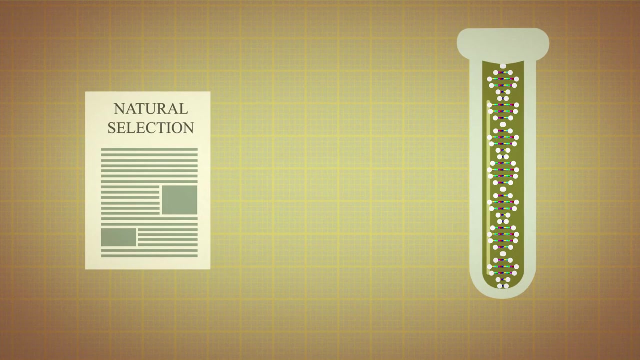 Charles Darwin published his theory of evolution in a book called On the Origin of Species. Extrapolating the theory of natural selection and combining it with discoveries made by modern genetics allows scientists to assert that all life on our planet came from a common ancestor that existed about 3.5 billion. 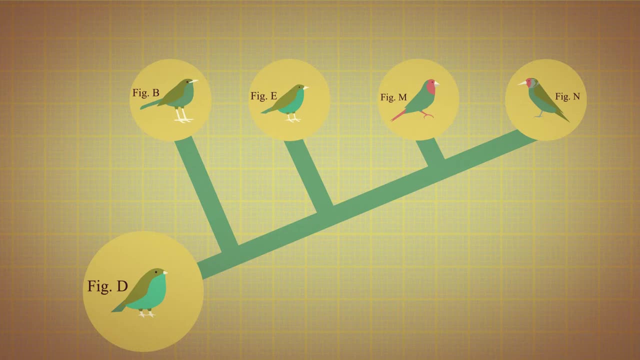 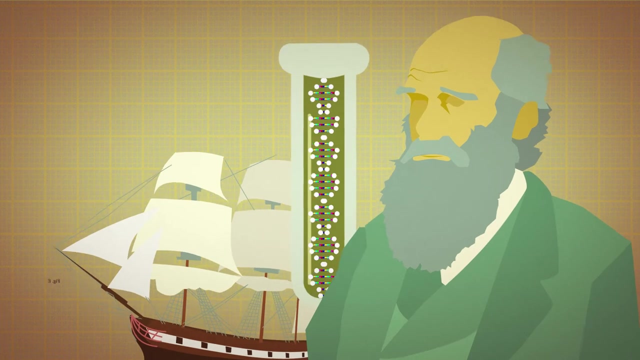 years ago. Through natural selection, new species are formed, Some species change and some are lost through extinction. In this video, you have learned that the voyages and research of Charles Darwin played a pivotal role in developing a theory about the origins of life and its variations on our planet, and that 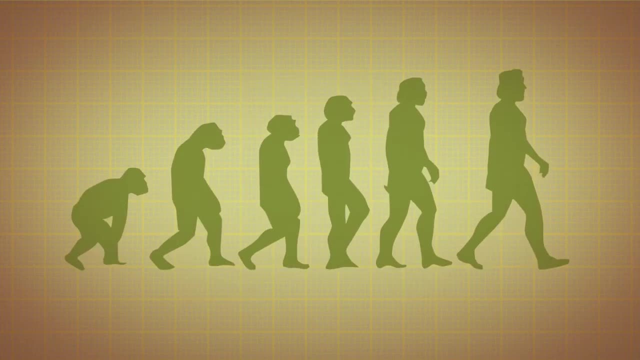 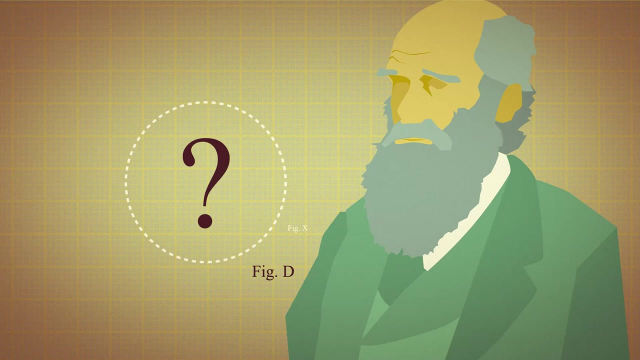 evolution is a fundamental part of our life. It is a process of continual change within a species as a result of chance occurrences. What else can you find out about Darwin? If you liked the video, give it a thumbs up and don't forget to subscribe. Comment. 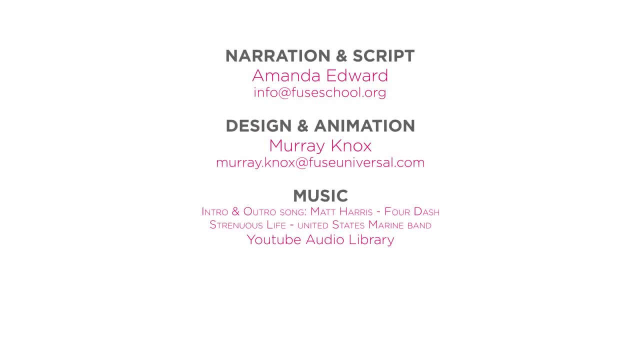 below if you have any questions. Why not check out our Fusco app as well? Until next time,